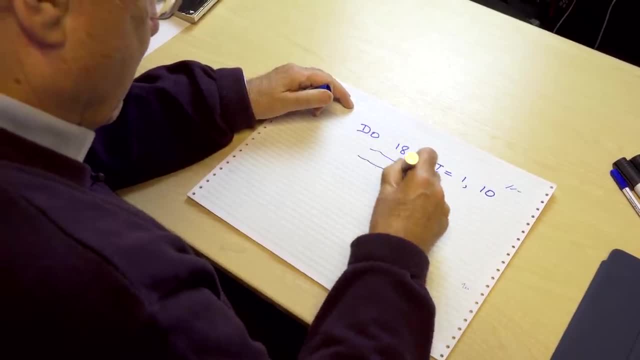 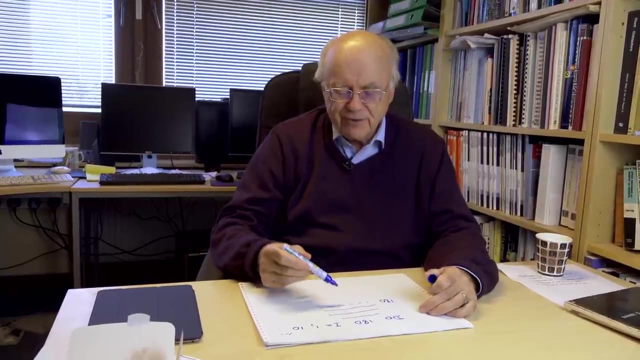 but not quite. They didn't call them for loops, they called them do loops. What I'm saying here is: you package all this up where you're saying: repeat the following sequence of instructions, which I've done with my wavy lines here: Keep doing them until. 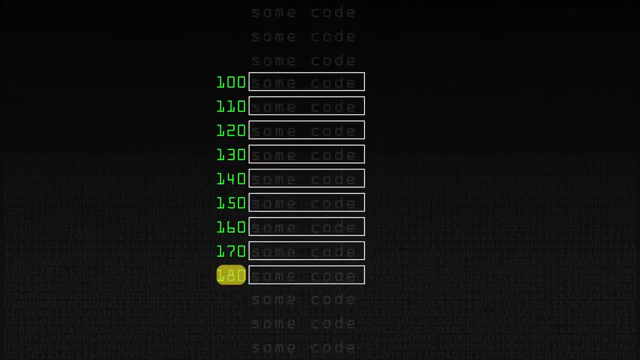 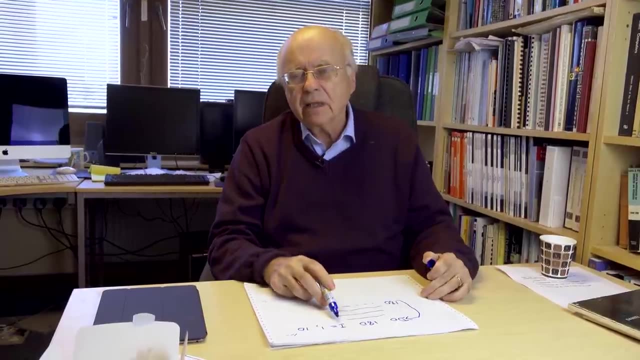 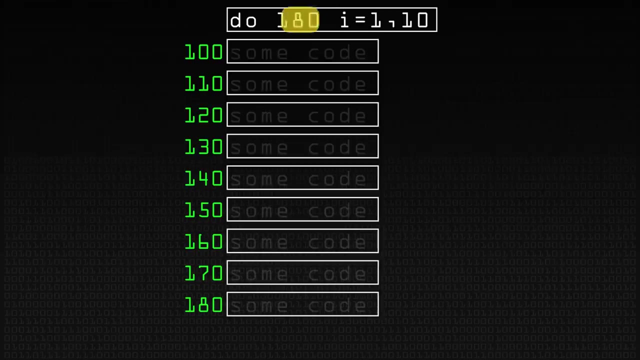 you hit the statement with a numeric label on it of 180.. The loop back from the statement labelled 180, back up to here to increment the loop counter which you're all familiar with in languages other than C. It wasn't done as it would. 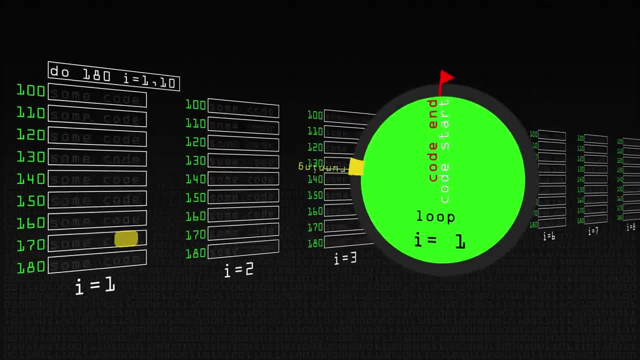 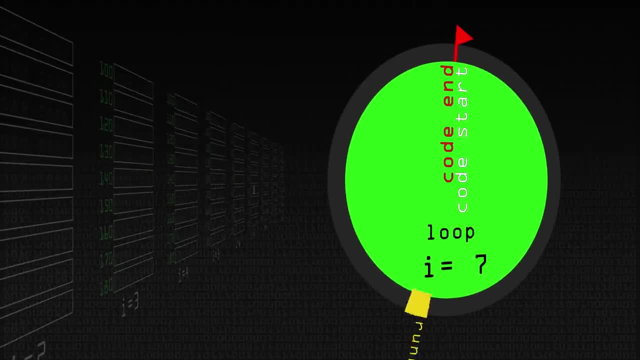 be in C by saying: here's my block of stuff to be repeated. It's inside these curly braces. Here you can see it's a lot more like Assembler, a lot more low level. I mean, there's nothing magic about 180.. It could be 72. It depended on your. 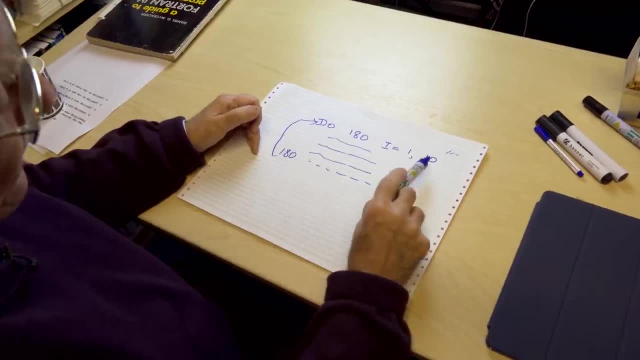 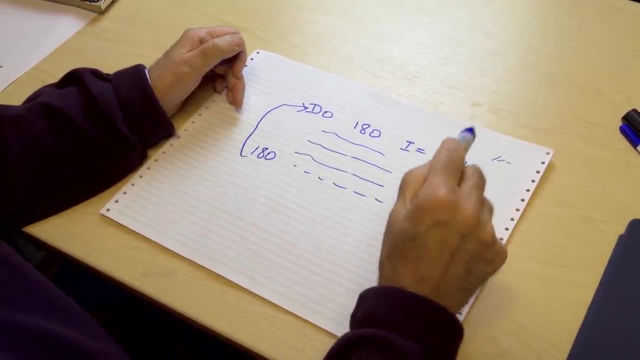 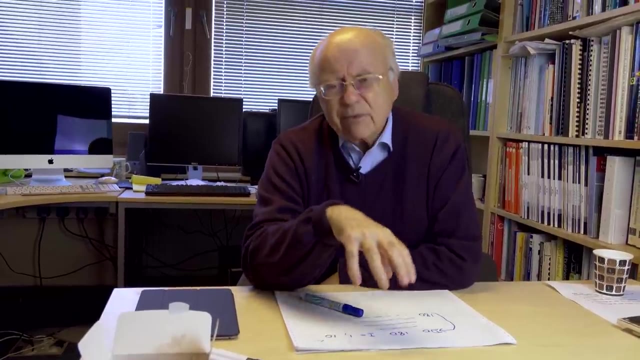 it would reset i to be 2,, 3,, 4, so on up to and including 10.. It's comforting for those who were coming from Assembler into high-level language to see something that was only slightly higher level in sophistication than Assembler was. 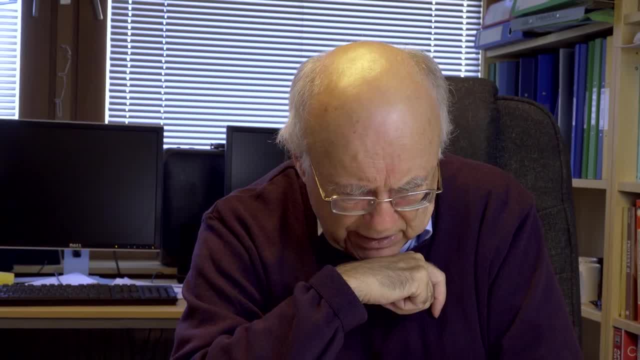 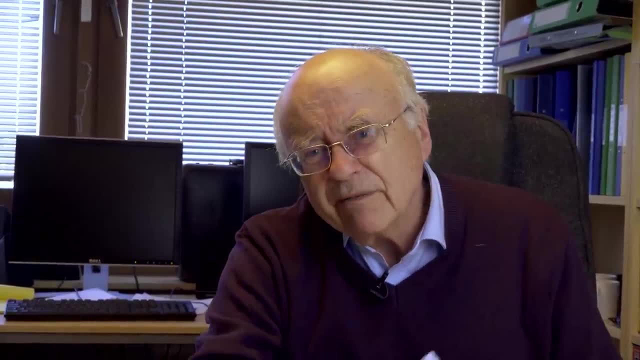 How did loops become more powerful, if you like? Well, again, even in Assembler and even in Fortran, there's no reason why you couldn't have a loop within a loop, So I might have outside of all this code. yet 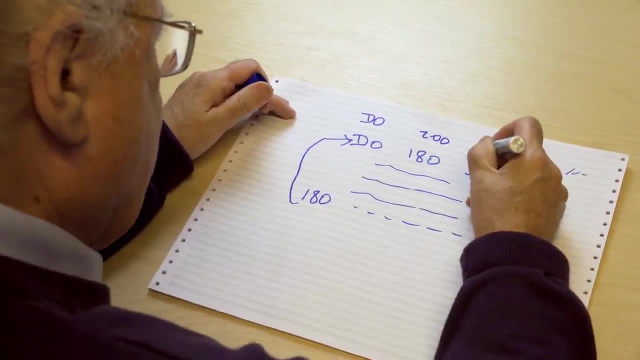 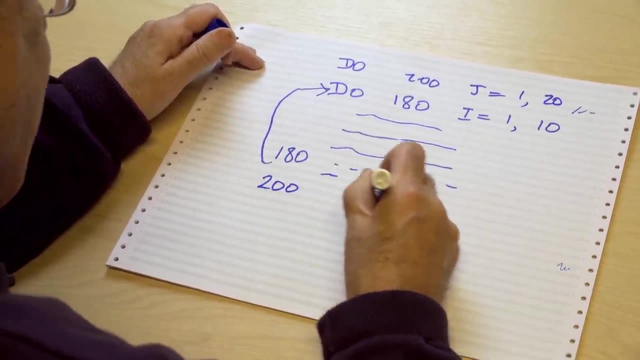 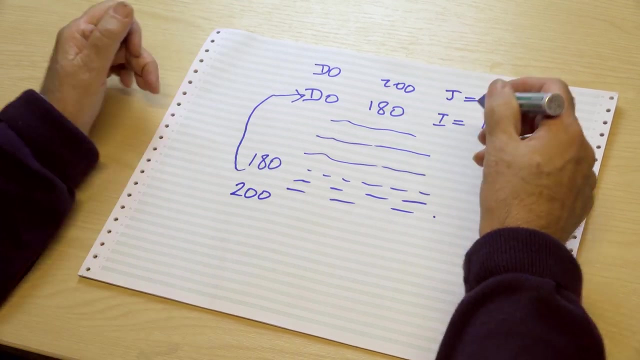 another layer of do What shall we say? 200.. j equals 1 comma 20.. So there might be some more statements between 180 and 200.. Who knows? But again you see a numeric label And can you see what's happening? Is that for every setting of j? 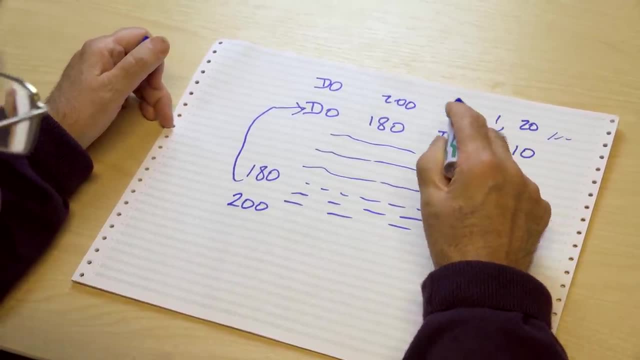 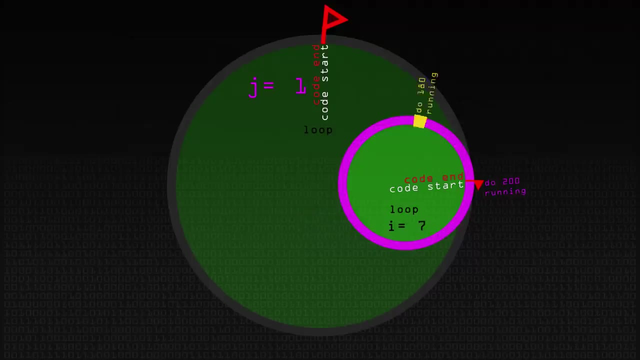 which will start at 1 and go up to 20,. for every single one of those j settings, the inner loop will be running through the complete spectrum of settings of i, going from 1 to 10.. So you will have 200 locations are being affected here. 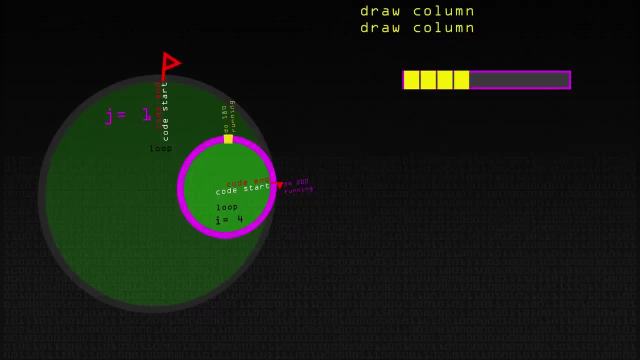 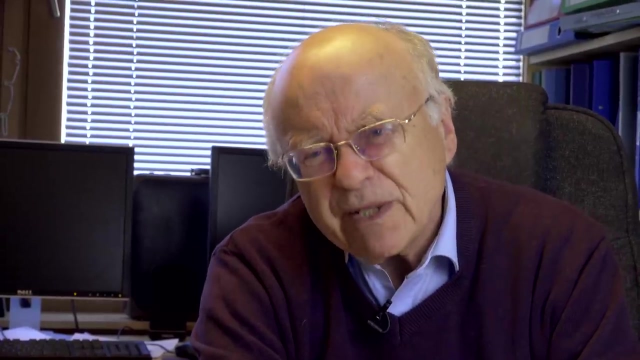 basically going through the rows and columns of a matrix. All sorts of calculations in physics, chemistry and particularly engineering just rely on two-dimensional arrays full of numbers, either integers or scientific numbers with a decimal point, and so on. Even hardcore Assembler pros had to admit if 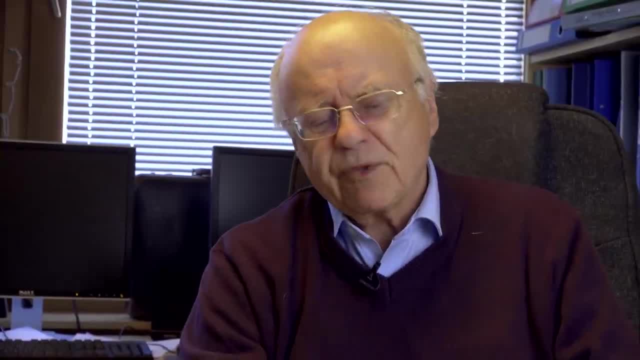 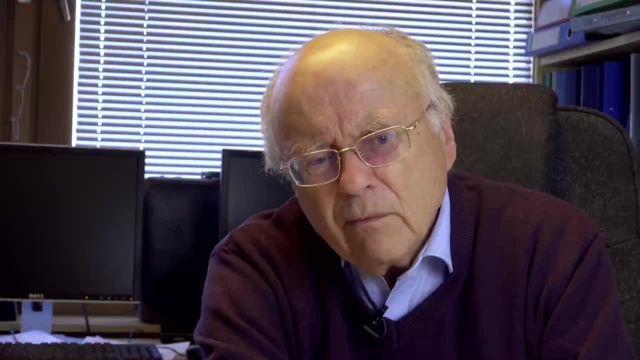 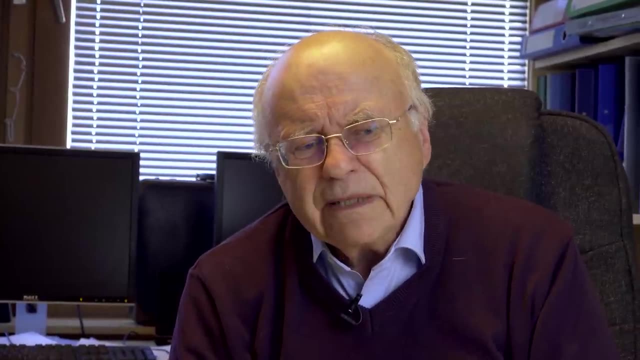 you were doing heavy scientific programming, it was nice to be a little bit more abstract and to have this sort of facility available to you. Now. you might say: well, what came along to spoil the party then? Or how did people realize that this was wonderful, but not quite enough? The compiler, of course, has got to. 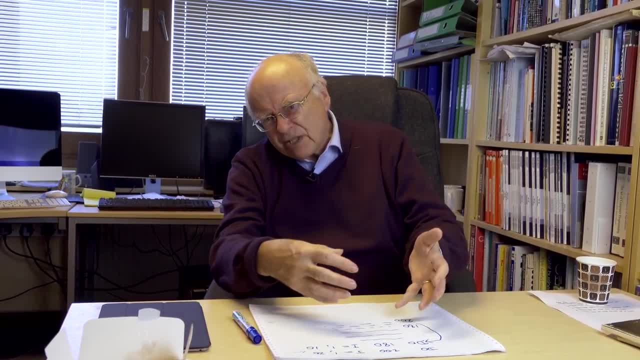 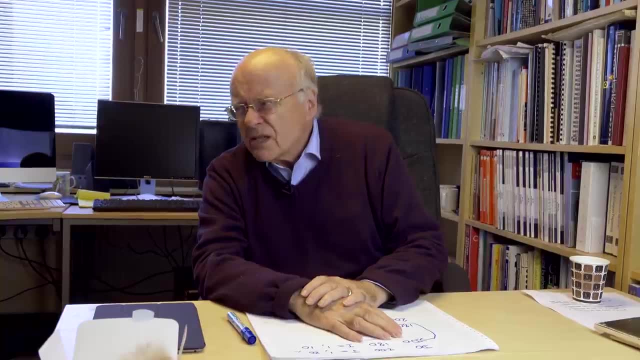 be tolerant and has got to be capable of compiling nested do loops correctly. But how deep would it? let you nest them? Well, I'm guessing. I would suspect that the early Fortran compilers probably wouldn't allow it to go more than about. 10 deep maximum And I think you and I, Sean, have just been looking up what are the current limits in C. I seem to remember the earliest GCC was something like 32, but I think we looked up that some C++ nowadays allows you to do. 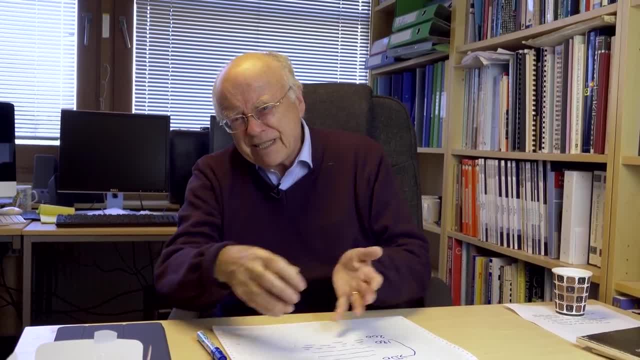 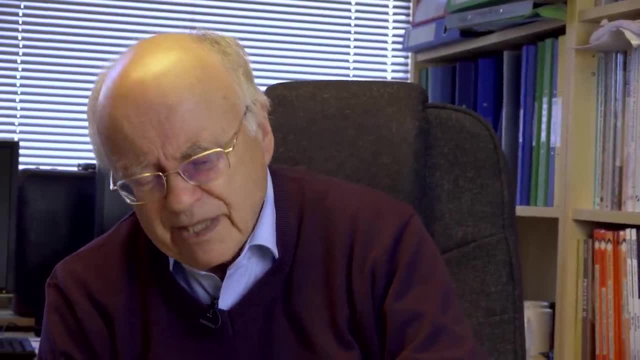 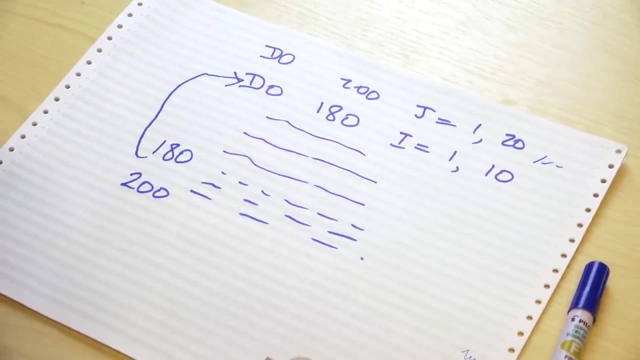 nested loops 256 deep, And of course there are multi-dimensionals problems that might actually need that, because it doesn't take much knowledge of higher maths to realize You've got a loop within a loop. The outer loop goes around n times. The inner loop is going around n times You are then coping with. 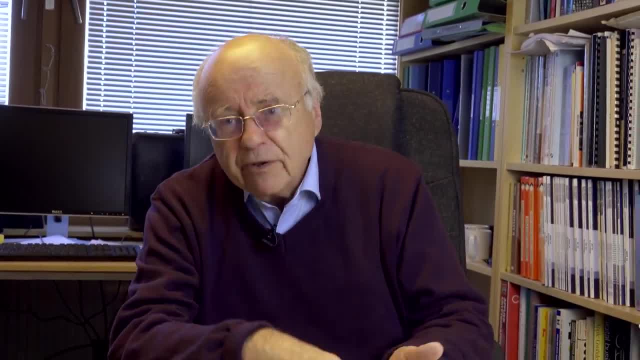 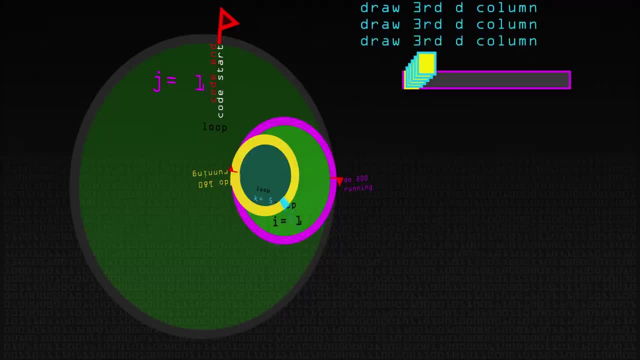 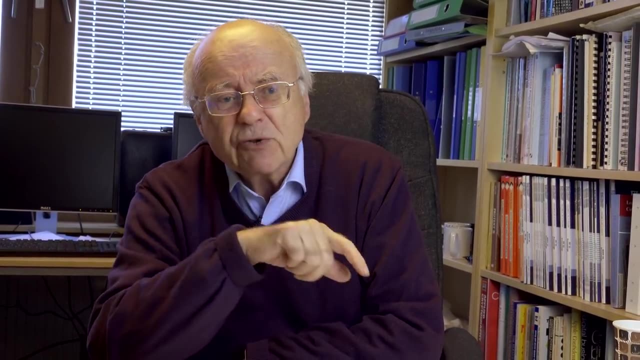 an n-squared problem. If you put the third loop inside the other two, you're coping with a cubic three-dimensional problem. So what we're saying is: all these multi-dimensional polynomial on exponential problems that come up quite naturally, you can cope with them. 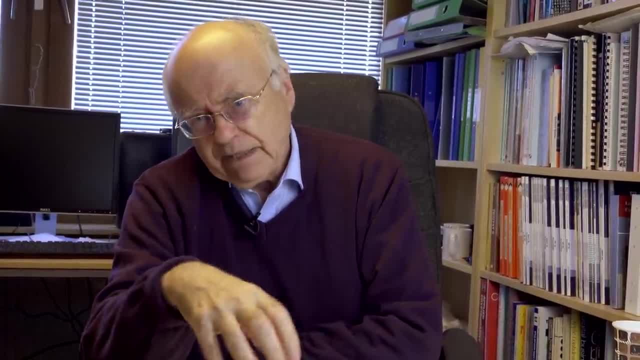 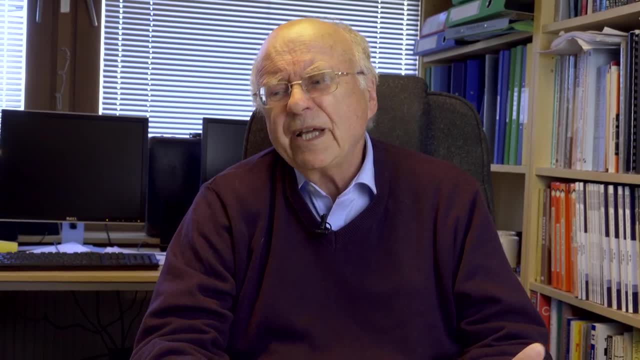 in nested for loops, so long as they don't need to be more than power 30 or power 256 or whatever it is, And you think, well, that should be enough for anybody. There's these multi-dimensional problems. You can just do them by nesting. 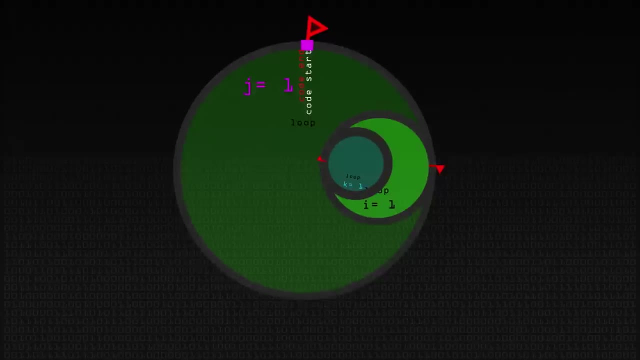 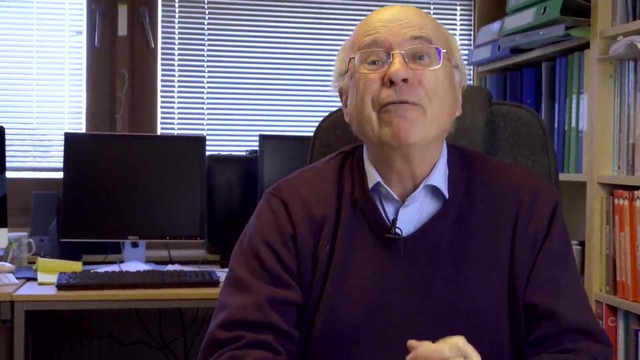 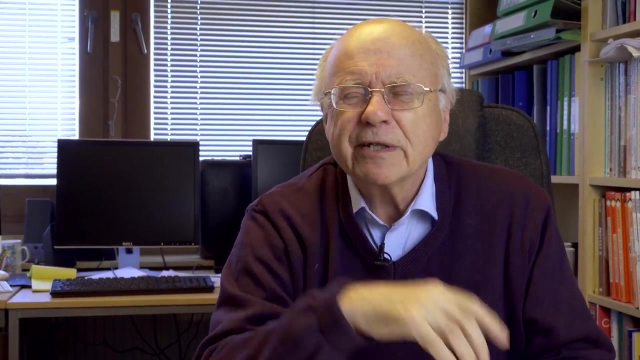 for loops, And surely 256 is enough for anybody. What kind of problem wouldn't it be enough for? Well, a lot of theoretical computer scientists of my knowledge amuse me greatly when those of them that will own up to this. back in the 60s, People started going to lectures from 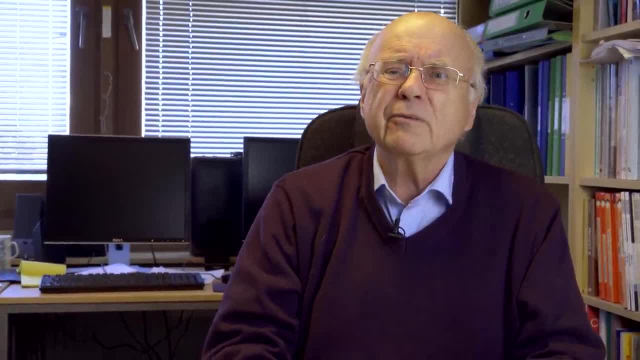 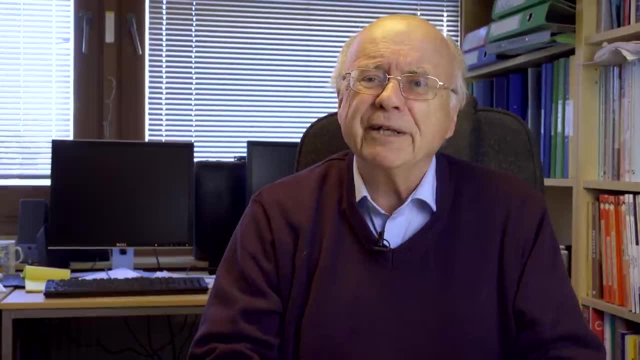 mathematicians, theoreticians, people concerned with girdle computability and so on, And of course those sort of people were very familiar indeed at a mathematical level with Ackermann's function. Now, as you know, you and I are, 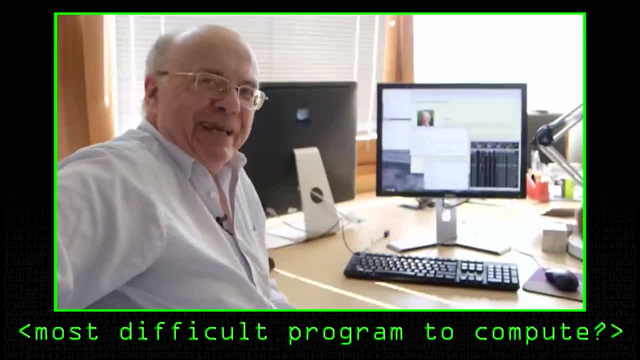 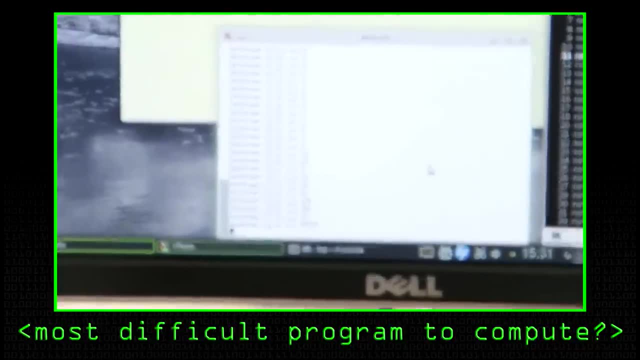 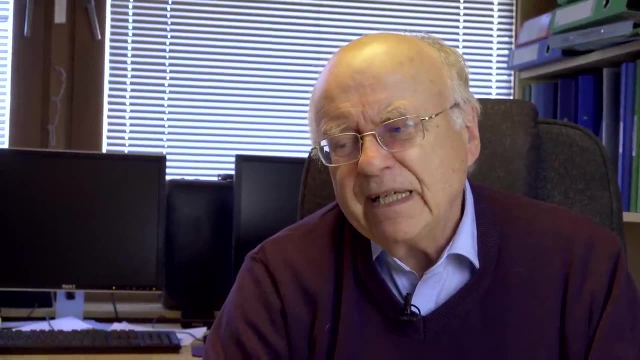 all familiar with algebra. We've done that once. Is that the most difficult, The most difficult number to compute? We set this going four weeks ago. nearly now The first few have vanished off the top. So what made it so difficult? Well, you write down Ackermann's function and it very clearly ends up with: 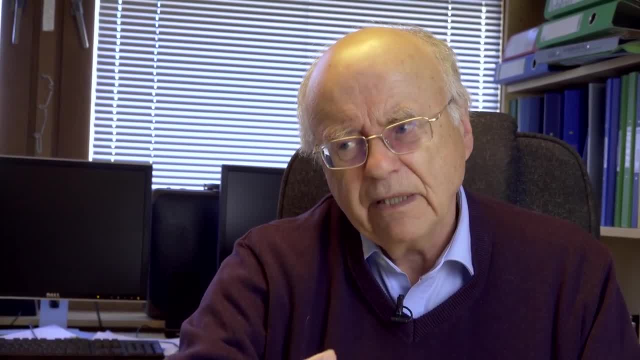 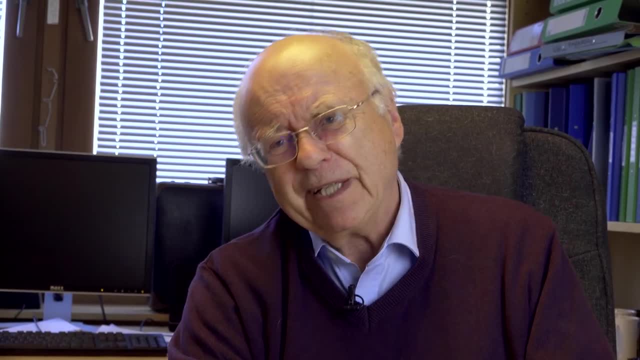 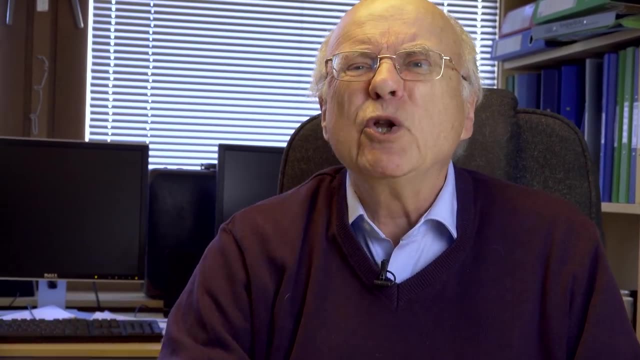 routines calling themselves recursively in a very, very complicated way. Now, I think your average sort of engineer would be happy to say that there's this thing called factorial, which is five times four times three times, two times one or whatever, and you could do that in a loop as well as doing. 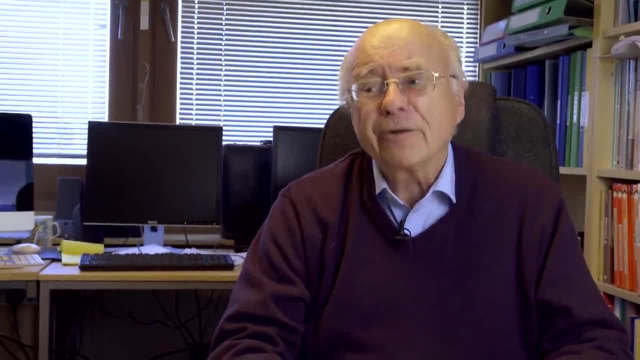 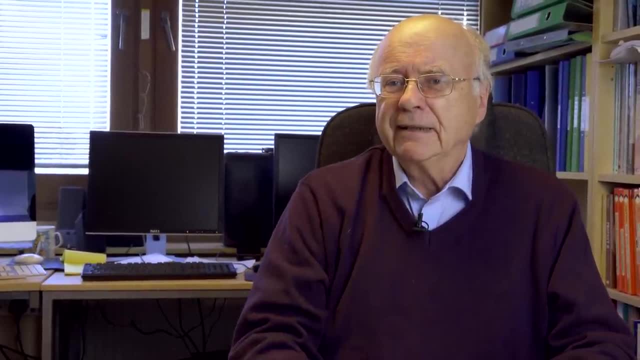 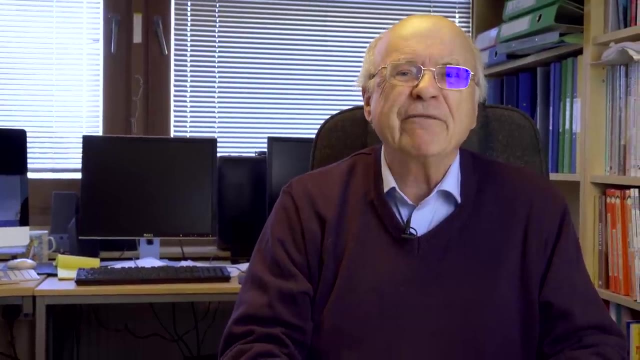 this fancy recursion thing. But a lot of theoreticians admitted to me. they saw Ackermann's function and said I could try that out in Fortran. Now, what they perhaps didn't realize- but it became famous by 1960- is: Fortran is wonderful. 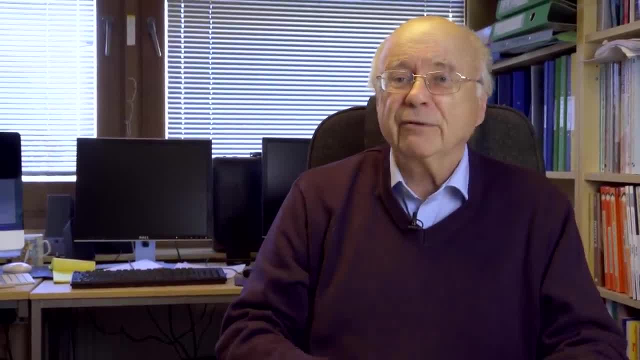 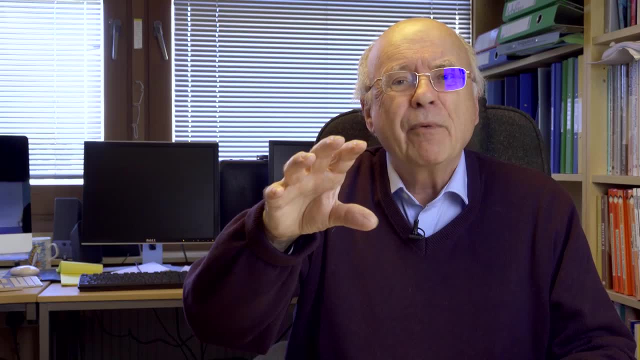 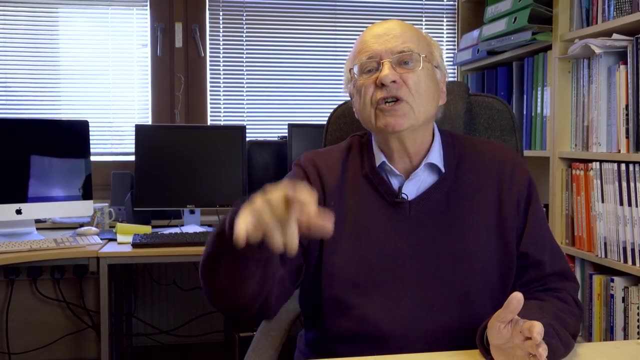 but original Fortran did not do user-level recursion. You could write a thing called Ack- You could actually get it to call itself in Fortran- But you might have been expecting that every time it called itself it would lay out a data area for each recursive call. They're called stack frames. We know that. 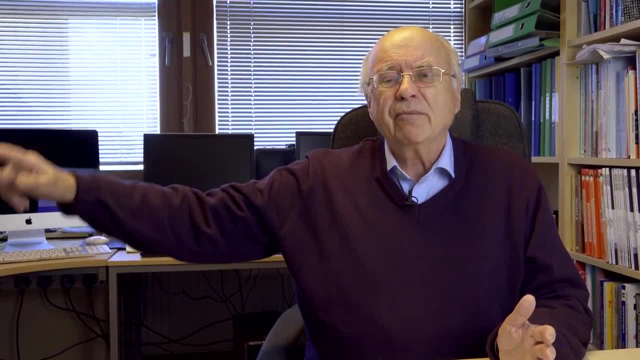 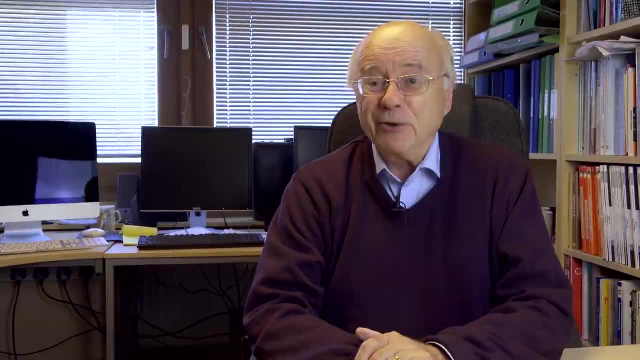 now You get lots of stack frames one on top of another, and as you come back through the recursion they're deleted and thrown away and you climb back into your main program. Fortran doesn't do that. It sets aside one stack frame. You keep calling. 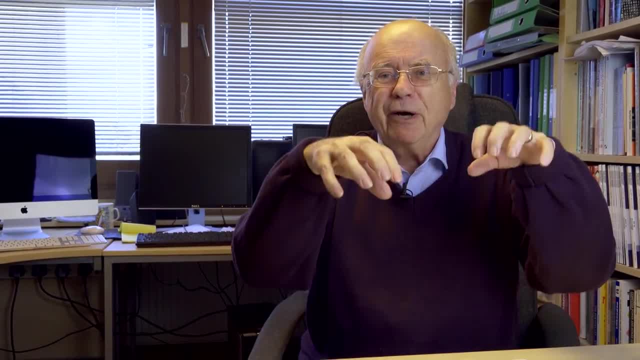 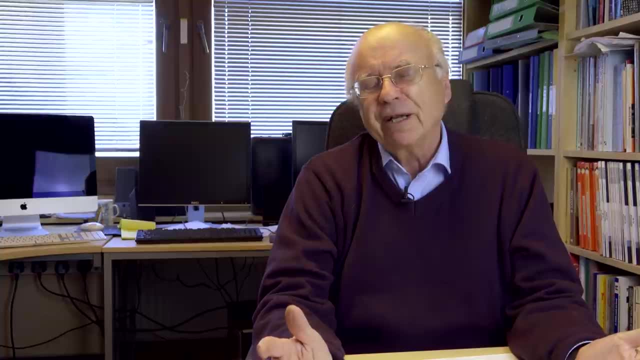 yourself recursively. it just tramples and it's muddy gumboots over all your data area and you end up with total garbage. It no more gives you values of Ackermann's function than fly to the moon. So people said, you know? I then realized the importance of 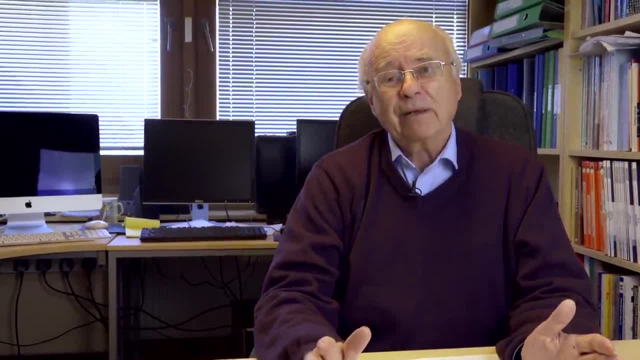 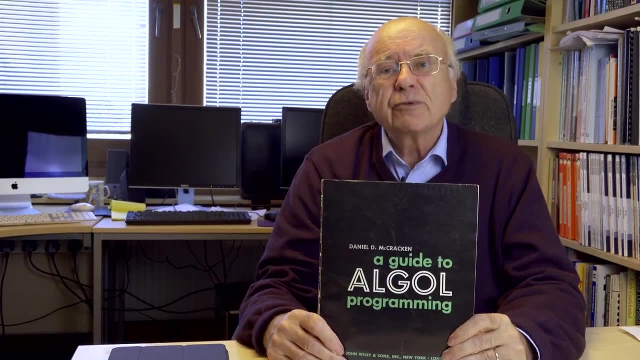 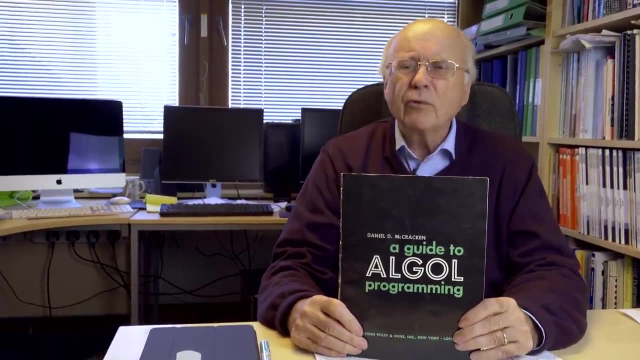 having user-level recursion in programming languages to cope with those really hard problems that fell outside. nested in Fortran, Algor was famous in that its routines could call themselves recursively and could get the right answer, And for limited low-order values of Ackermann's. 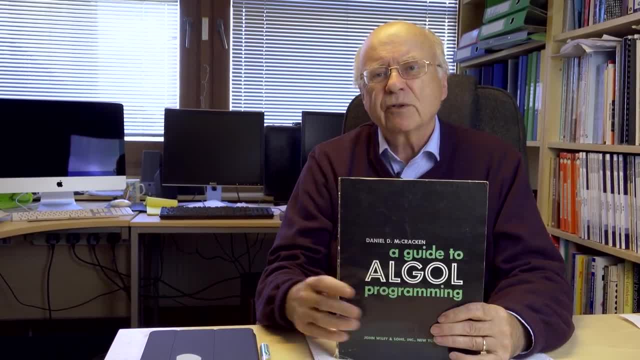 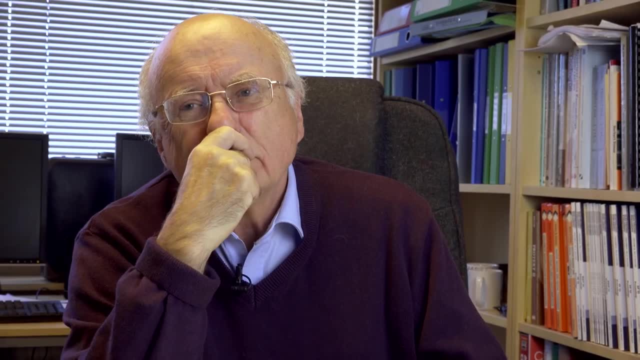 function Very slow, very slow indeed, but it would come out with a right answer. Is there an easy-to-think-of example of a problem or program? Because Ackermann feels to me like it's. it's like the test bed, you know when you're testing out a motorcar. 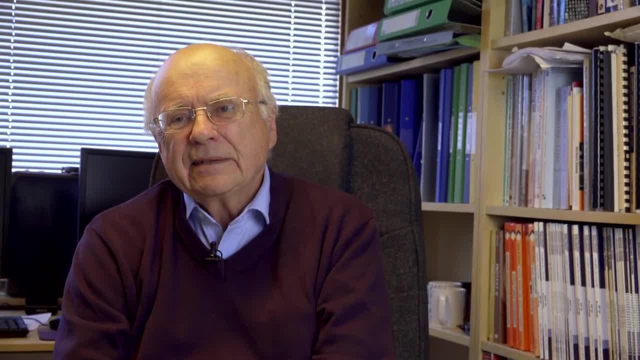 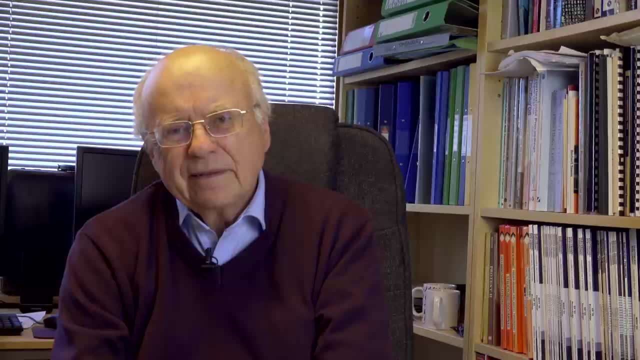 You might take it on the track and see how fast it can go, But in day-to-day life that car might only get half that speed. Yeah, What's the real-world kind of equivalent? Is there such a thing, Real-world equivalent Of something that might need to use? 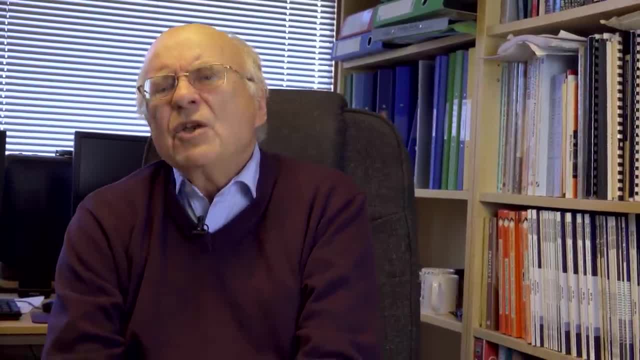 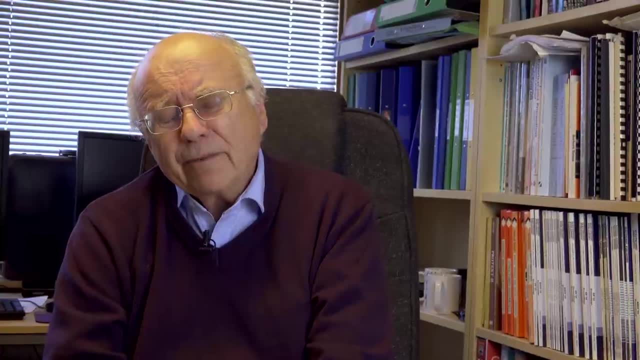 recursion. that Of that complexity- Not many things- is the answer to that. I mean. yes, it's true that Ackermann, as you know, was David Hilbert's research student and the challenge was on to find something that was so innately recursive. 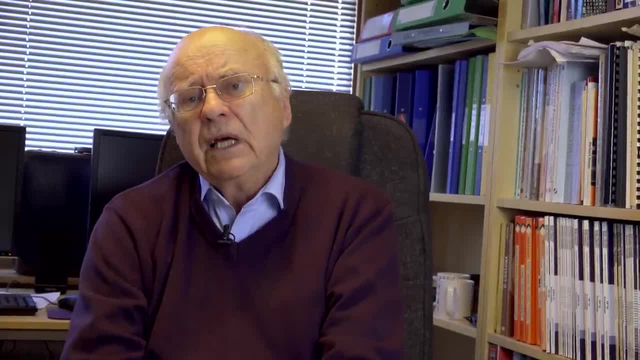 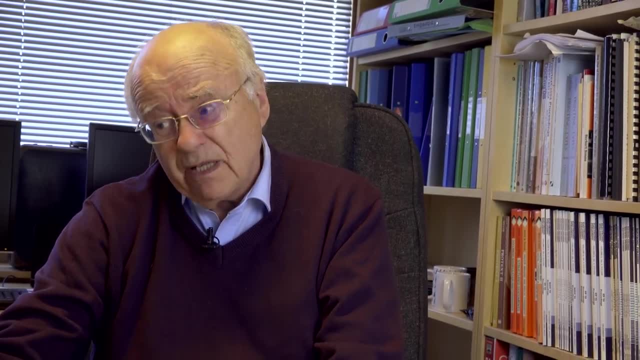 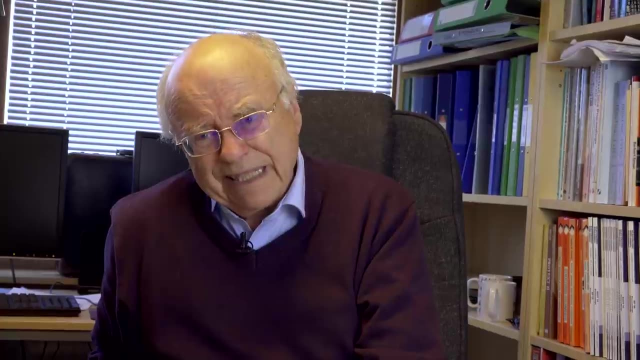 that you remember is sort of generally recursive they called it- As opposed to primitive recursive and simple things like factorial and you need Fibonacci are primitive recursive. So I think you're right that you really are just making the point that eventually there are things that will kill you, I think. 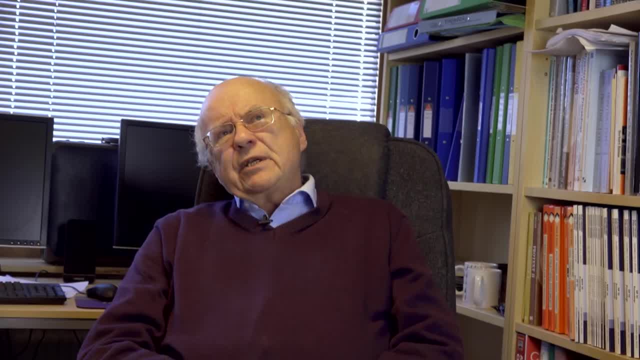 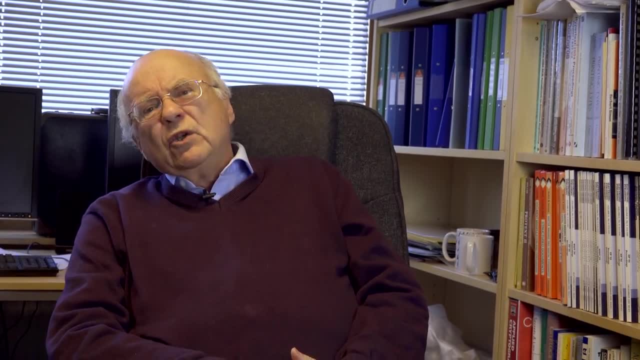 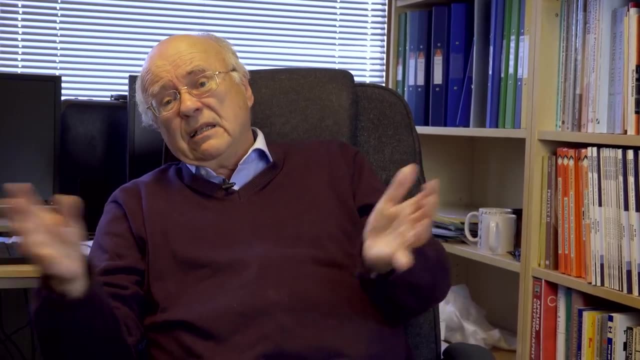 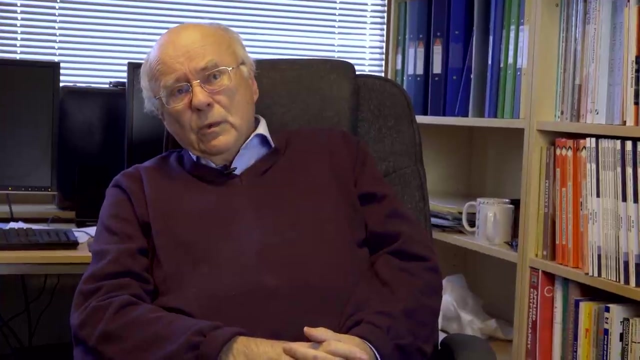 the. the question in the middle is: is there something, are there pieces of program you need to write, where non-trivial recursion in a sense is needed, but not quite to the horrendous degree that Ackermann did. And the answer is yes. Compilers is where it hit people Because, although early, 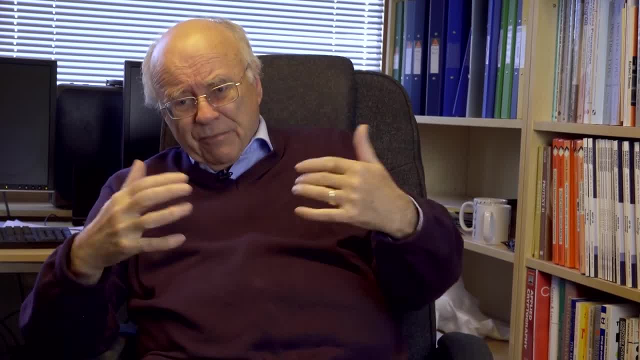 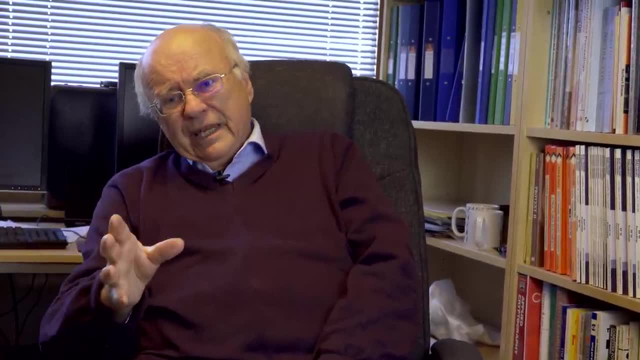 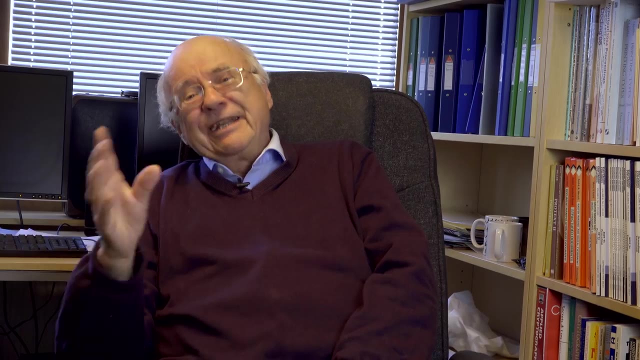 Fortran did not provide user-level recursion for you and me. nevertheless, John Backus and his team implemented it in the middle 1950s, I think, at IBM, And Backus wrote articles afterwards basically saying we didn't know enough about recursion and even though we didn't provide it for the 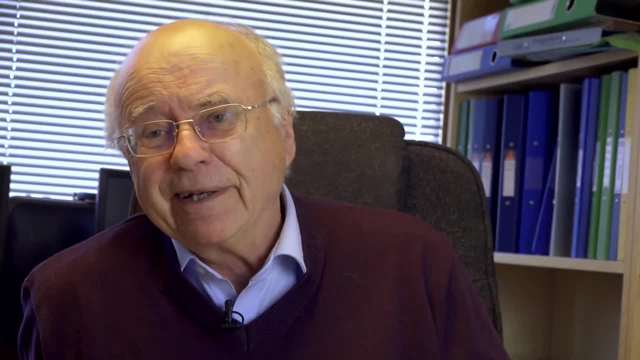 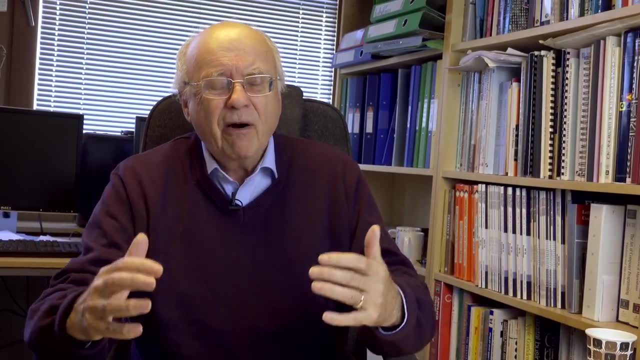 users of our language. boy did we need it in the compiler And we invented. we ended up inventing it in all but name The syntactic structures of what is legal in a language, even at the level just of arithmetic statements can be.